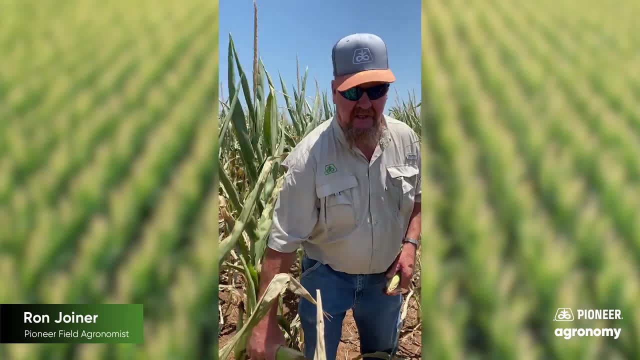 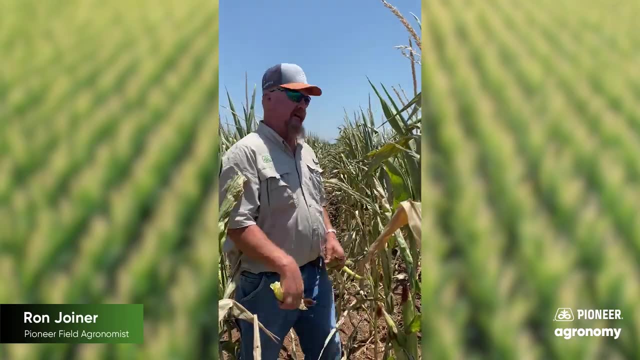 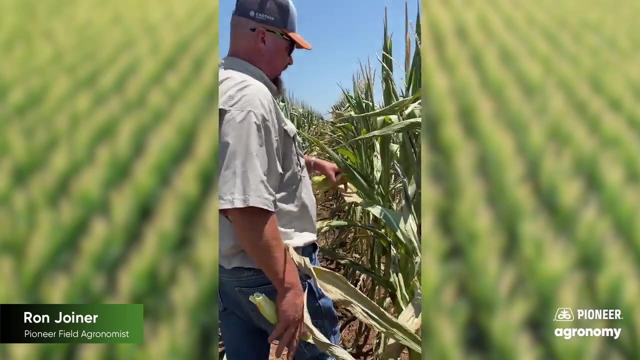 down Question I would have about this is: what kind of yield can I expect out of these particular plants, and will there even be any? Here's an air on down the row. Let's go on down here and see what it looks as we get across the field. Notice, as you go through here, a lot of these leaves are. 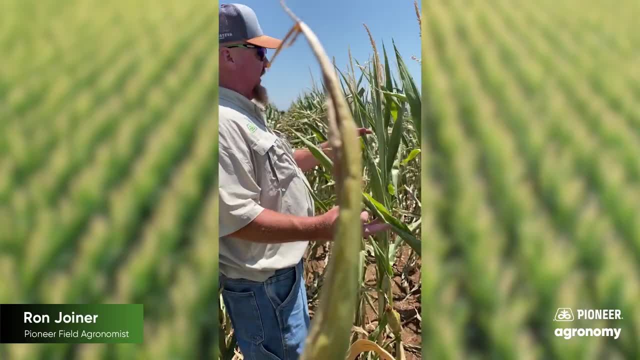 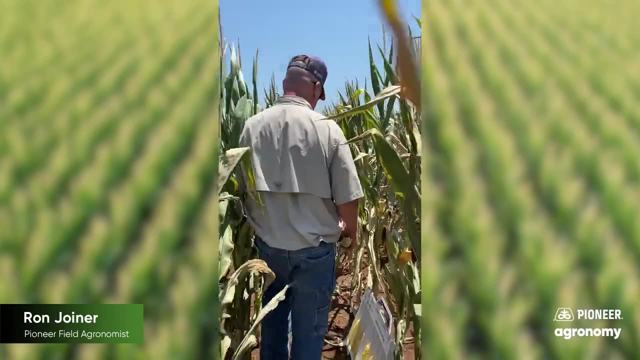 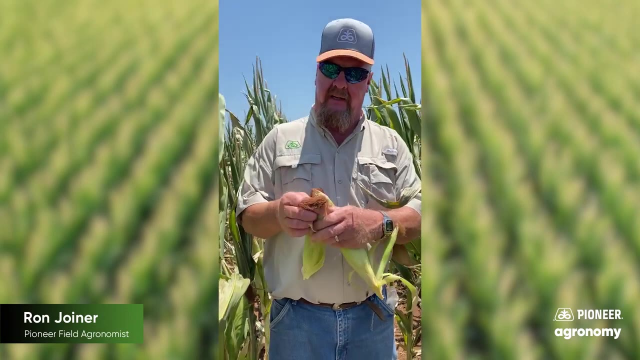 scorched very little photosynthesis happening. These are still alive, but severely rolled up, and of course the husks are starting to turn white. So as we look right here, it starts to improve as we get on down there. So we've got an ear that I pulled back there. Let's investigate. 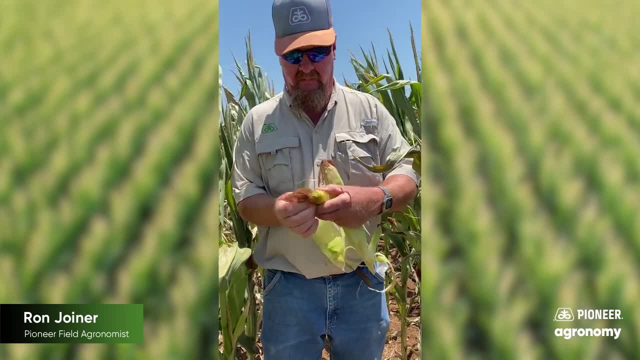 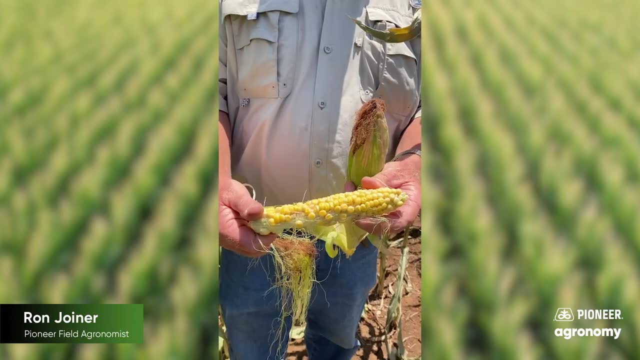 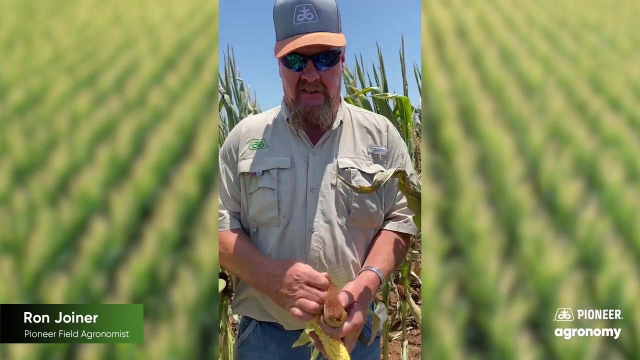 this a little bit and see what it looks like. Well, number one, you can tell right off the bat a little bit of incomplete pollination, probably due to drought, and that piece of soil is very, very shallow back there a lot of rock. This is an ear. 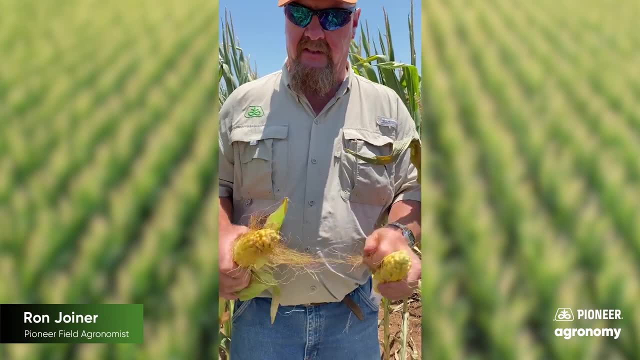 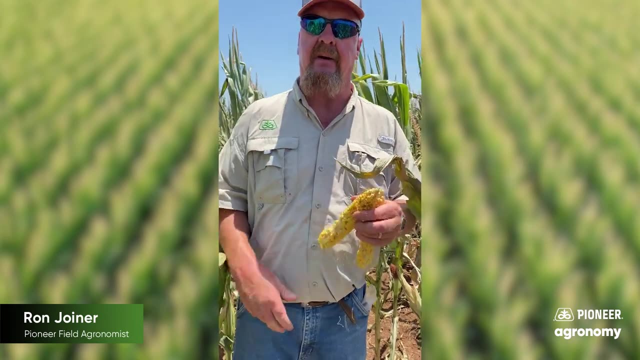 I pulled on down the way, It's a little better shape, but one of the things you'll notice is some missing kernels. My expectation here is probably that was a late roundup application. We had such severe dry weather early in the season. We didn't have any of that. We had a lot of dry weather. 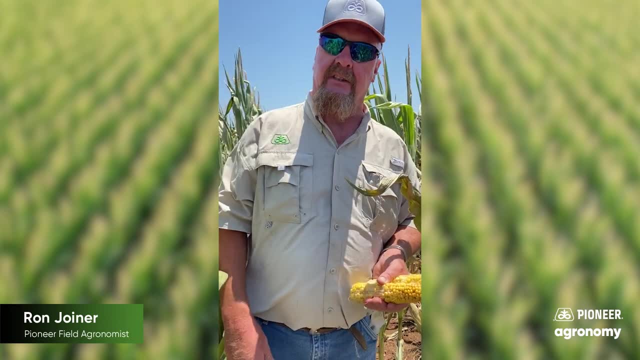 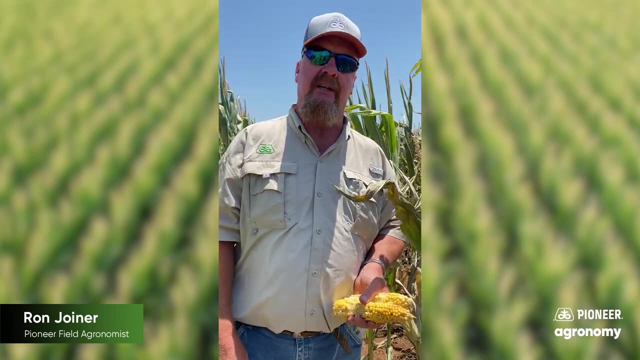 and we didn't have weeds to spray at the correct time. you know, V8 or 30 inches, whichever comes first, When you have a drought, a lot of times you shorten the internodes and you'll have plants at a farther growth stage than you ever imagined. So you could see, looking here, these ears are not. 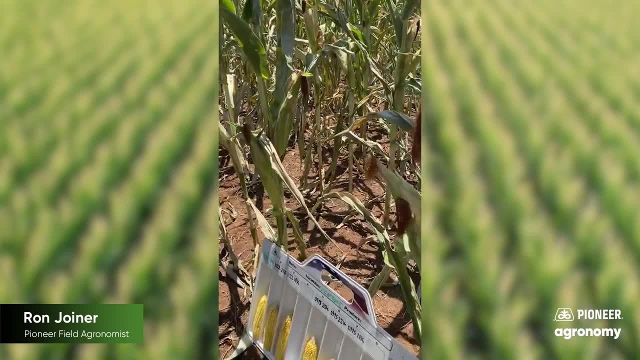 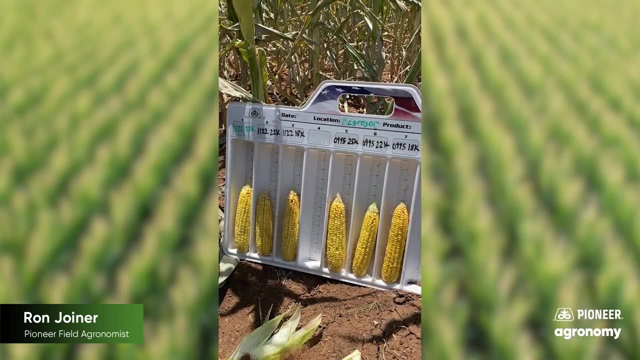 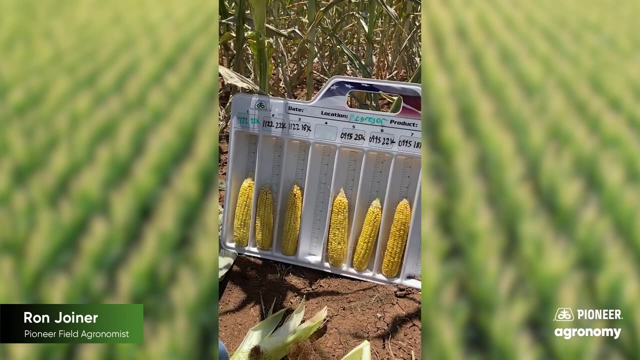 going to yield that well. But if you look down here at this board, where we've gathered two hybrids, two different ones- new 1122 and new 0995- at differing populations, they look pretty decent. It's a different part of the field, a little bit better soil And notice our populations: 25, 22,. 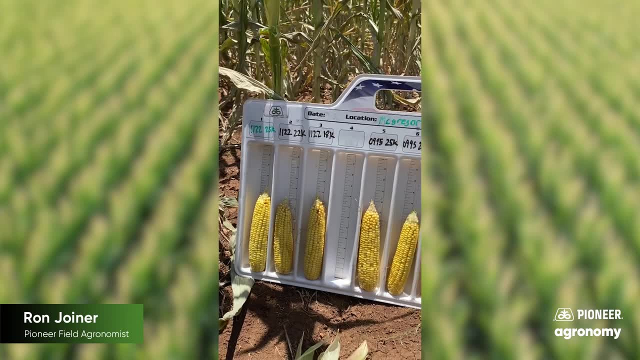 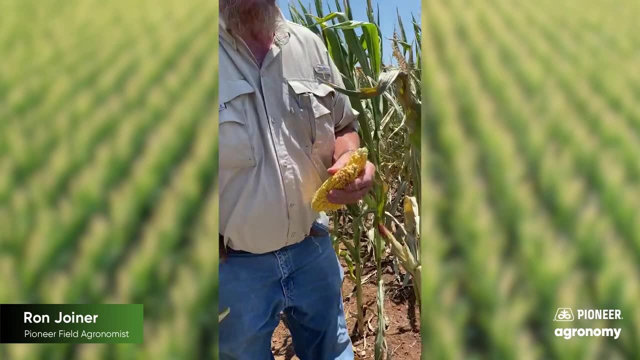 18.. So 25 on this piece of land is probably a little bit rich, 22 is probably about right and 18 is on the low side. So a question I would get is: okay, Ron, what's going to happen to these? 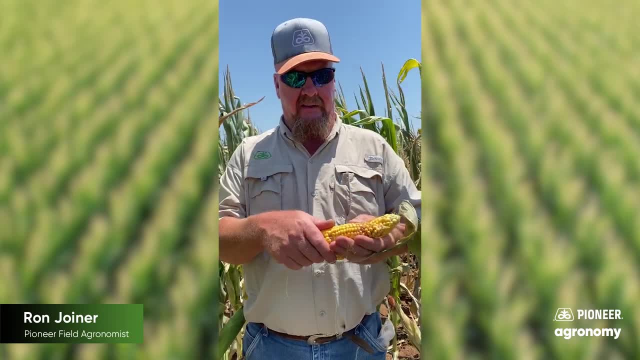 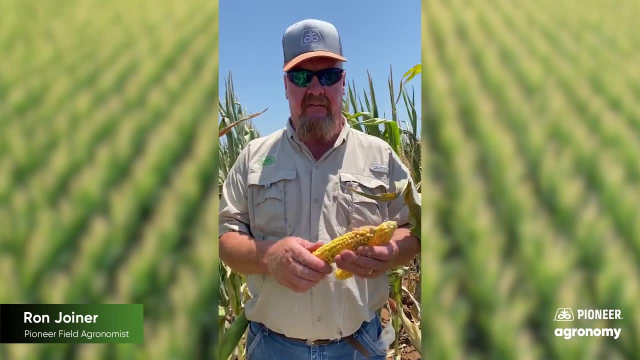 ears if these plants die. Well, we're at the dent stage for the most part, or early dent. You're not going to abort kernels on the tip any longer because you're at that advanced growth stage. What you will see, though, is you will see these kernels shrivel.